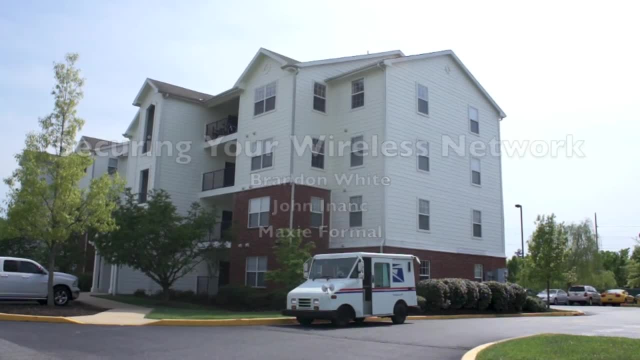 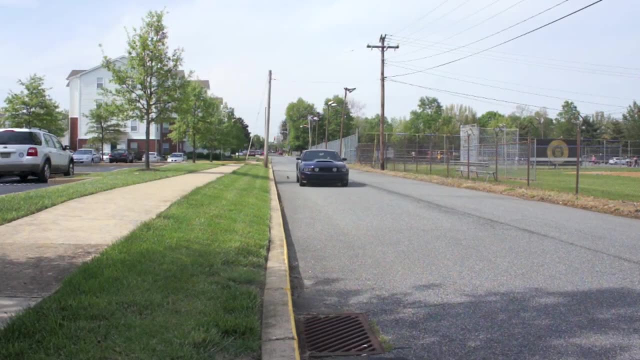 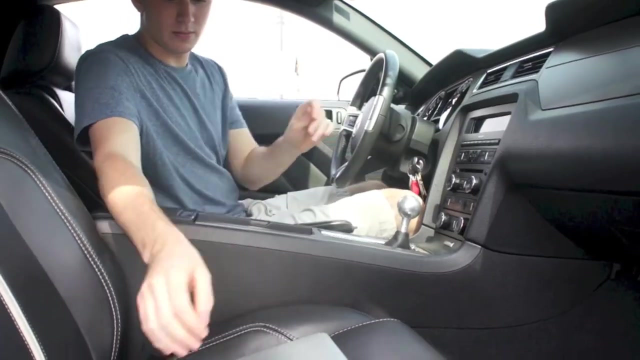 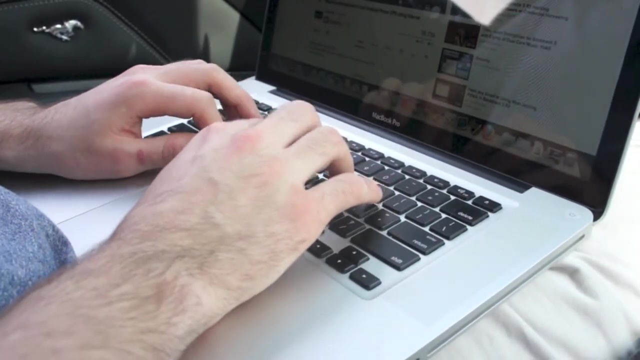 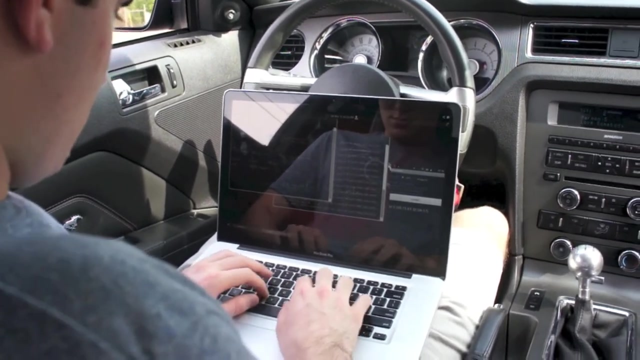 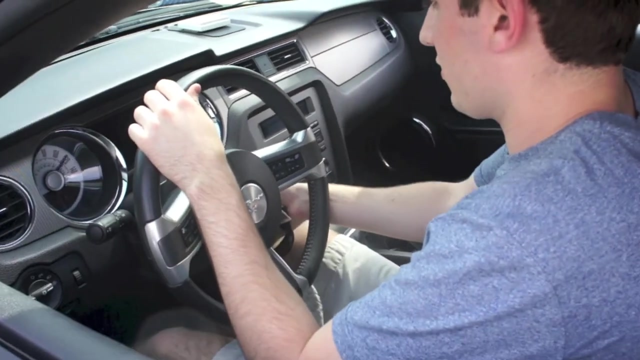 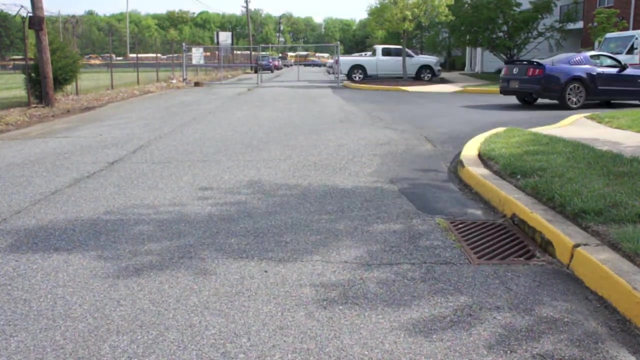 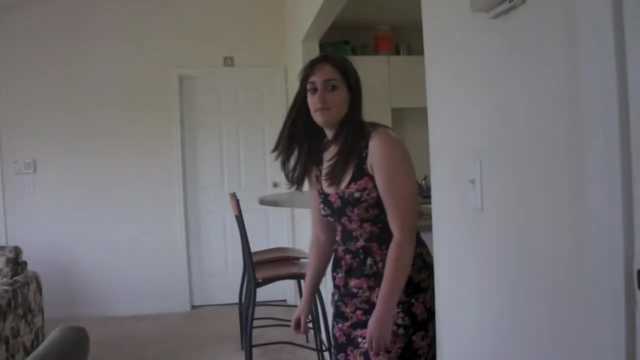 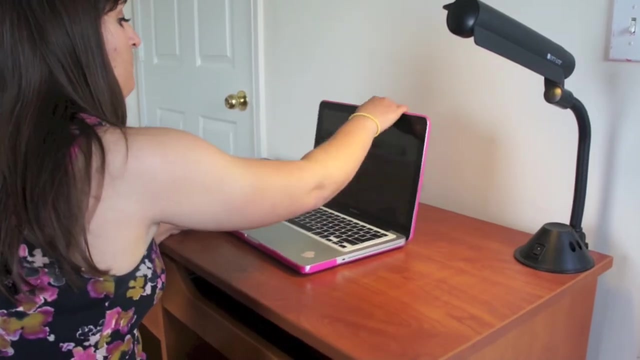 If you have any questions or other problems, please post them in the comments section of this video. If you have any questions or other problems, please post them in the comment section of this video. If you have any questions or other problems, please post them in the comment section of this video. 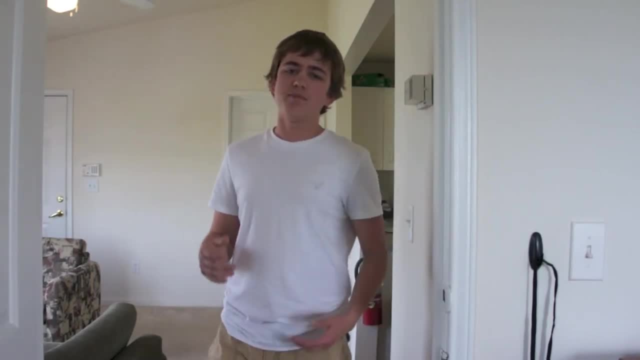 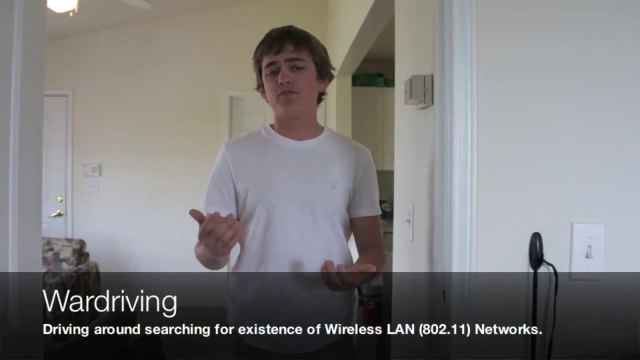 Maxi was a victim of identity theft because a hacker gained access into our computer by through a process of war driving. War driving is when a hacker drives around the neighborhood searching for wireless networks, and once he finds one with an unsecure wireless signal, he uses a. 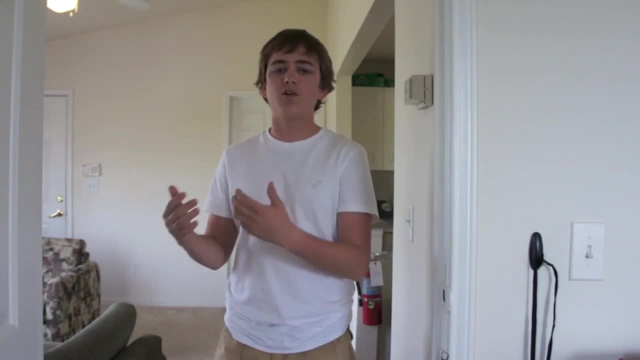 systematic process to hack into the wireless network and then gain access to all the internal computers and files within that network. In this case, Maxi's computer was completely compromised and her identity was stolen, leaving her with nothing. This computer was compromised because Maxi was using an unsecure wireless network. Today, we're going to show you how to set up and. 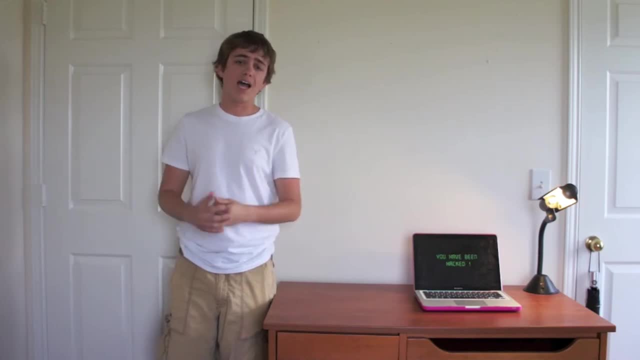 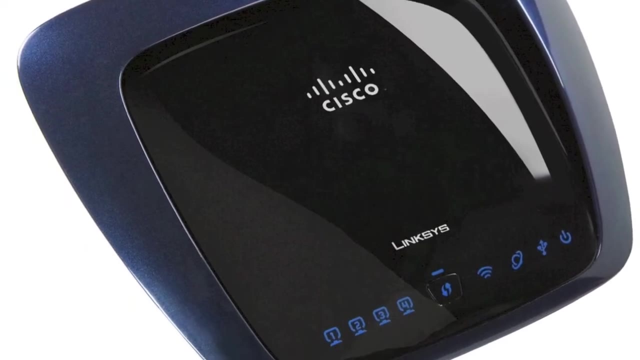 secure your wireless network. to make sure what happened to Maxi does not happen to you, The first thing you want to do is set up your router. In order to set up your router, please refer to the installation guide that comes with the router after you purchase it. Normally, it will involve: 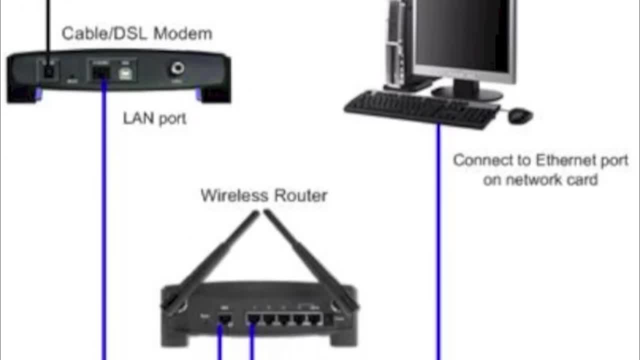 you hooking it up to a cable modem and then plugging in your devices to the back of the router, to which you will then use an installation CD to set up the basic configuration of the router. Once you've done that, you can go ahead and install the router. Once you've done that, 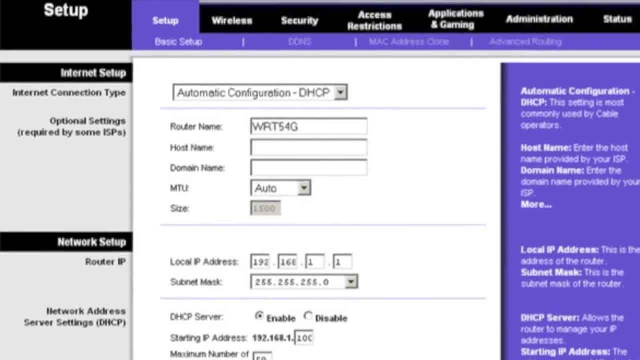 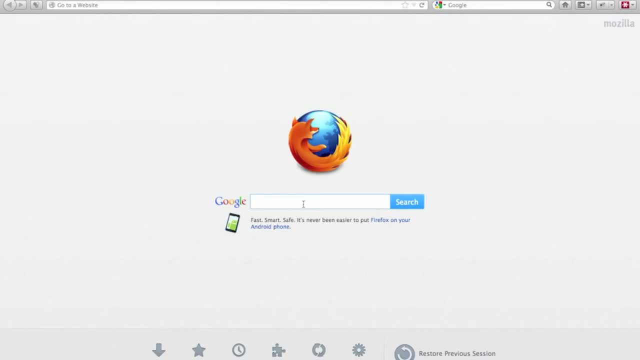 you can now move on to step two, which will show you how to set up a secure wireless network. So now that you have your router set up, let's go ahead and log into the back end of the router. The first thing you want to do is open up your web browser. I'm using Firefox in this example. 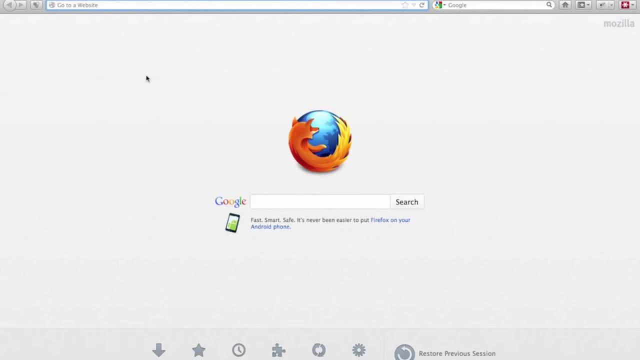 and you want to go over to the address bar and type in the access IP address of your router. This is usually printed in the router handbook or on the router itself. I'm using a Linksys router, so the IP address for me is HTTP colon- forward slash, forward slash. 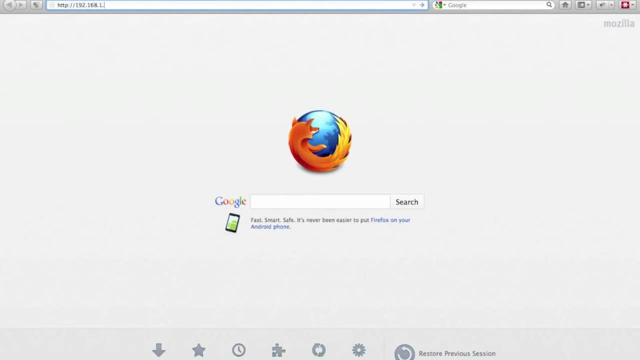 192.168.1.1.. Yours may be different or may be the same. Hit enter and you'll be presented with a login screen. This is where you enter the username and password. This is also going to be printed on the router and or in the handbook. There's many different variations. 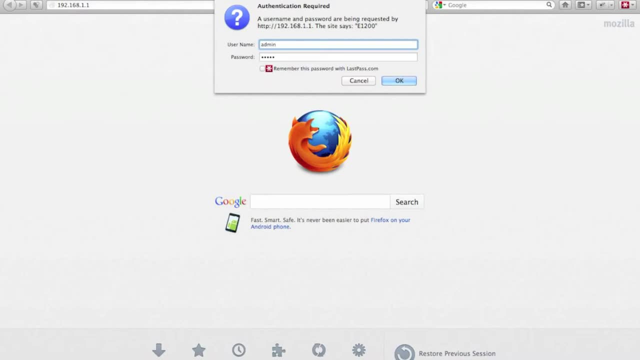 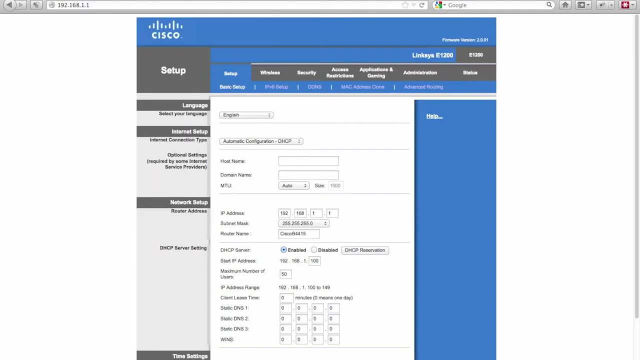 for the default access. It could be admin, admin, admin password, admin password one. There's a couple of different variations, So put that information in, hit enter, and now you're going to be presented with the splash screen. We're actually inside the router's configuration right now. A lot of this stuff is going to 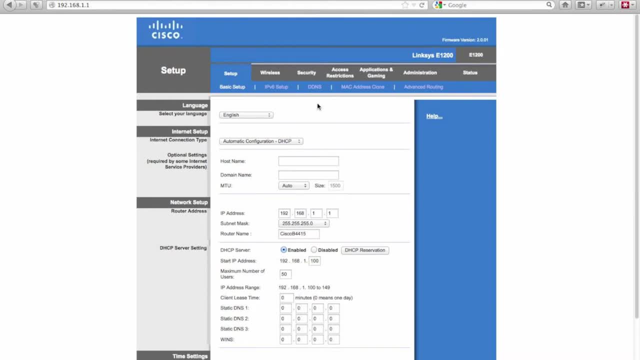 be set up when you purchase the router. You can either do that by using the handbook or the installation CD that comes with the router. But for the purposes of this demo, we're going to show you how to just set up a wireless network. 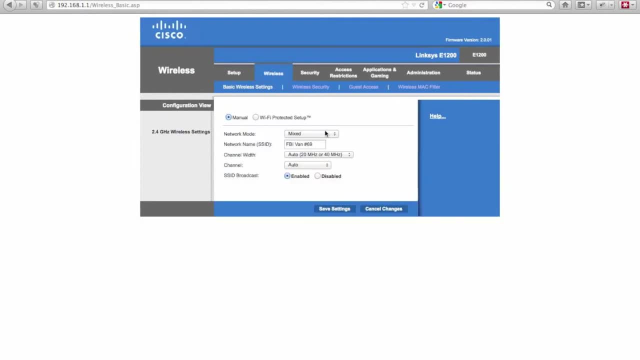 So what you want to do is click on wireless, And this is for Cisco routers. NETGEAR routers might look a little different than this, but it's all the same general concept. Find the wireless tab and you'll usually be pretty similar to how our Cisco routers look like. 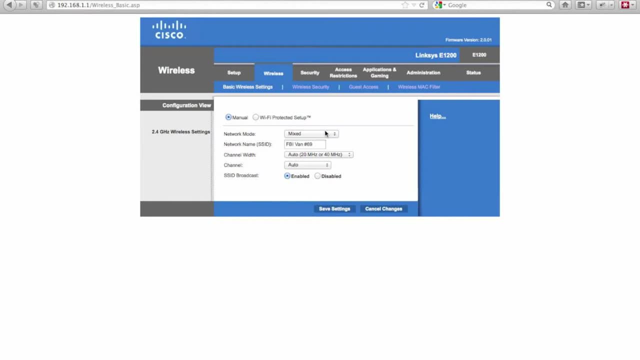 And you'll notice that we're on the basic wireless settings page right now And you'll see we have network mode, network name, channel, width, channel and SSID broadcast. We're really just going to focus on the SSID and the SSID broadcast on this page. But if you want, if 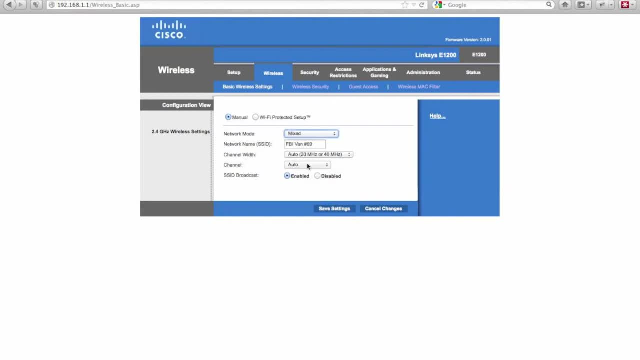 yours are anything different than this, I would recommend putting them on mixed auto and auto, And the reason I would put it on mixed is because it allows you to utilize all the different standards of the 802.11,, A, B, G and N wireless access points. So you'll. 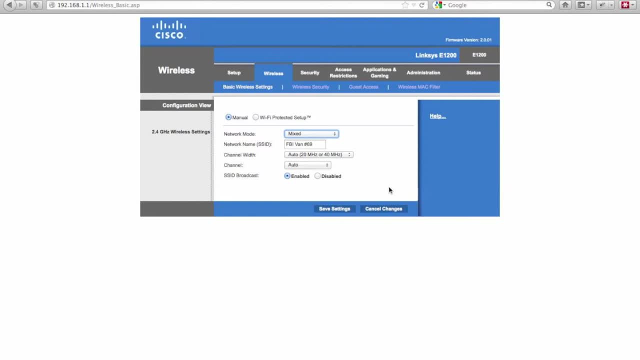 be able to connect to a wide variety of devices with a wide variety of speeds, And it lets you get a better broadcast out of the router itself. And the first thing you want to do. I already have a wireless network set up, but you want to type in the name of your wireless. 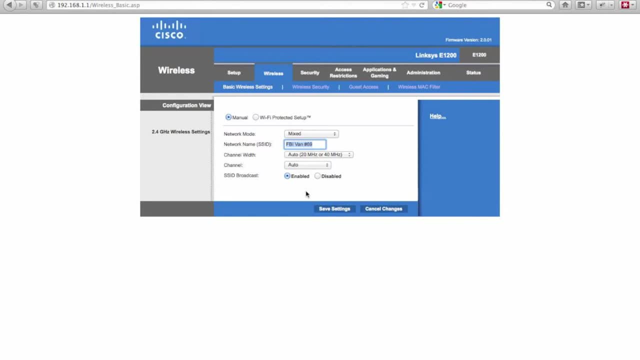 access point, which would be the name of the network that you're going to be using. So if we were to type in testing as our SSID and save this up here in the corner, when you go to connect to the wireless access point, testing would appear in this list of wireless. 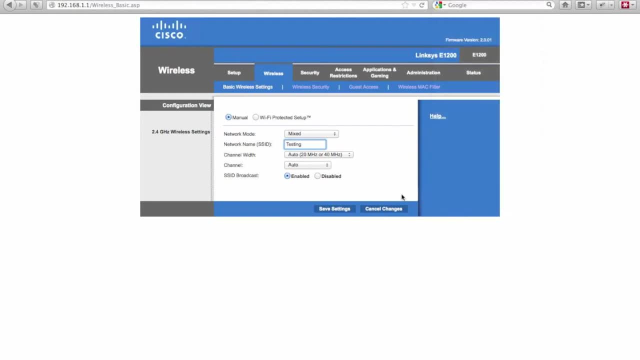 networks. So you type in the name of the network and that's what you're going to be connecting to, And then you can either choose to broadcast the SSID or not to broadcast it. If you choose not to broadcast it, it's not going to appear in this list. You would have to go to join. 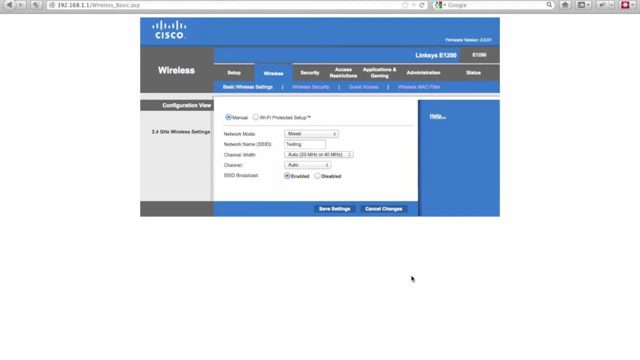 out of the network and type in the name manually and you'll have to connect to it. This is really just an extra layer of security, because it really helps prevent wardrivers or network sniffers or anything like that from gaining access to your network, because they won't. 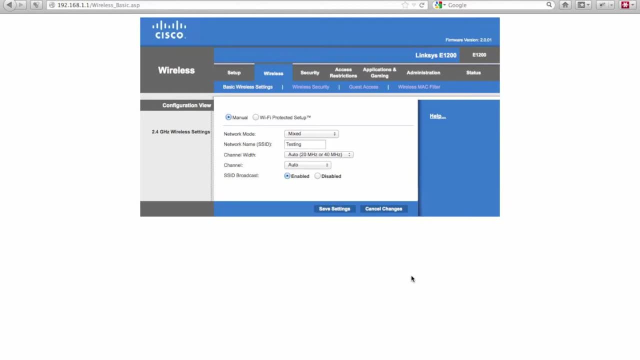 actually see the network. So there's a couple of ways to do that. So first off, you can see the network name and unless they can pick up like an encryption signal, there's no way that they would even be able to gain access to your network. But you know, I like to keep mine enabled only. 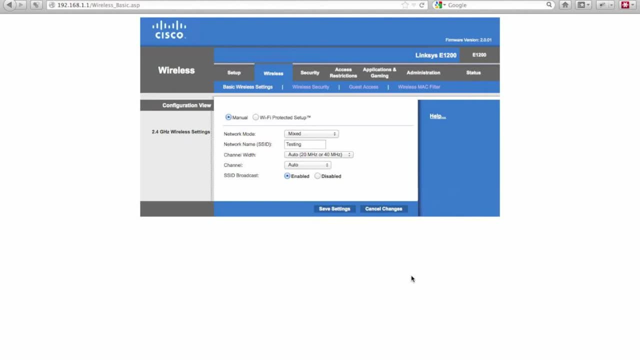 because I have guests that come over and it's a lot easier for me to connect up my Xbox or my iPhone or all those other devices without having to manually find the network and get into it. So we're going to keep ours as enabled, and then you would save those settings and then 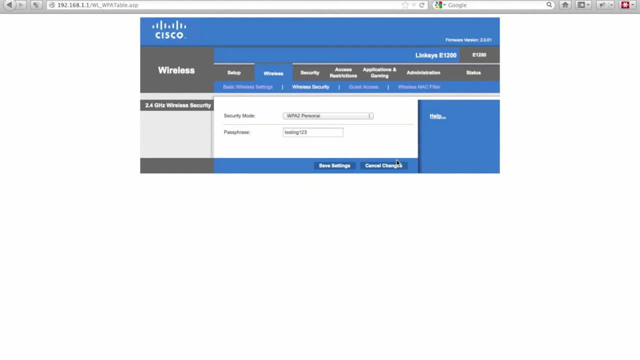 click on the wireless security tab. This is the most important part of the wireless security. if you drop down security mode, you'll notice that the router comes built in with a bunch of different preset logins- Really the two main networks that we focus on, or network security. 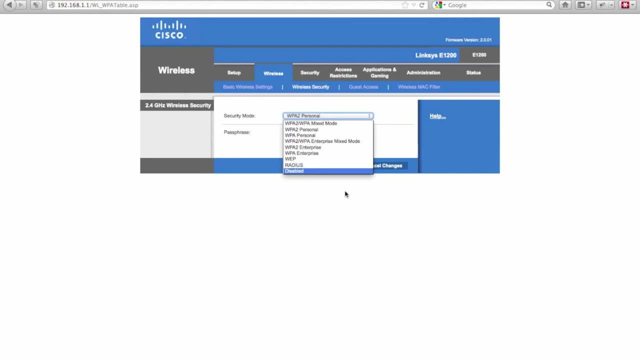 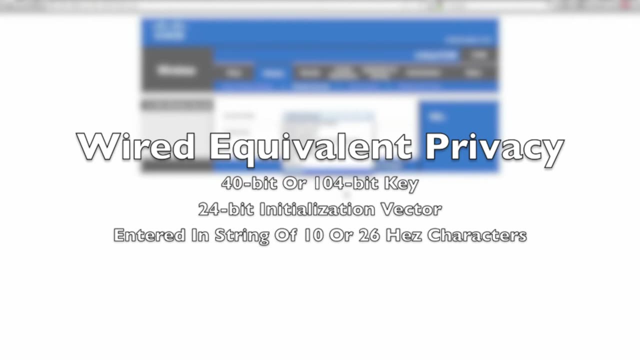 types that we focus on are WEP and WPA. WEP uses a RC4 streaming cipher to encrypt the data stream between a WLAN client and an access point. It uses a 40-bit or 104-bit key and combines that with the 24-bit initialization vector to get the seed for encryption. The key is shared between the. 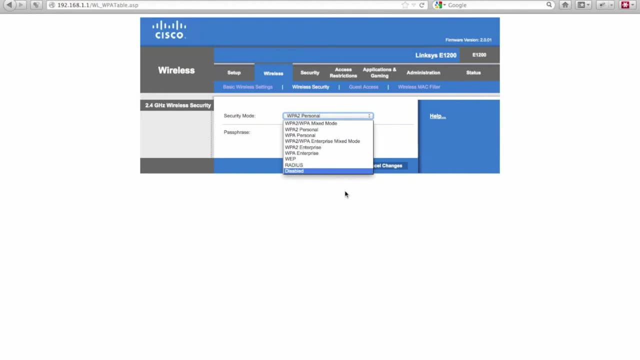 WLAN client and the access point, and it's usually entered at a string of 10 or 26 hex characters, And this can become a real hassle because this isn't really something that you can make up. It's more of a pre-generated key, just a bunch of different numbers and characters. You usually 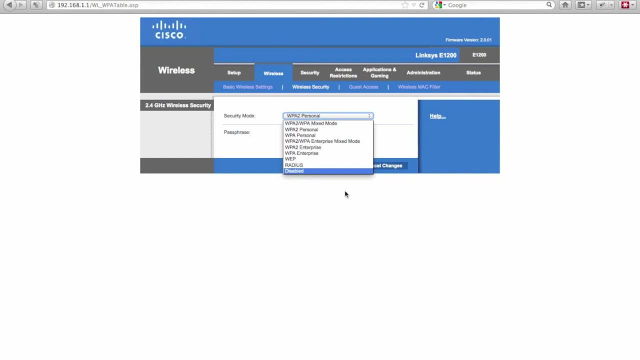 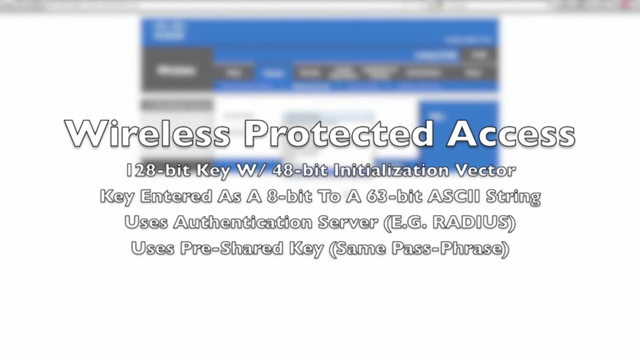 have to write this down And it's a real hassle when you have people come over and you have to go find it where it's written down at because you may not remember it. It could honestly become a real nuisance. Or you can use WPA2 or WPA- WPA is wireless protected access which also uses an RC4 streaming. 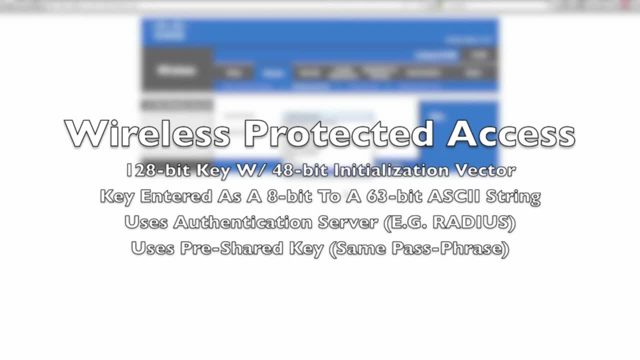 cipher to encrypt the data stream. but it uses 128-bit keys with a 48-bit initialization vector And you can input either an 8 to 63-bit ASCII string, which is just normal characters. your QWRTY1234 exclamation point: add symbol, stuff like that. 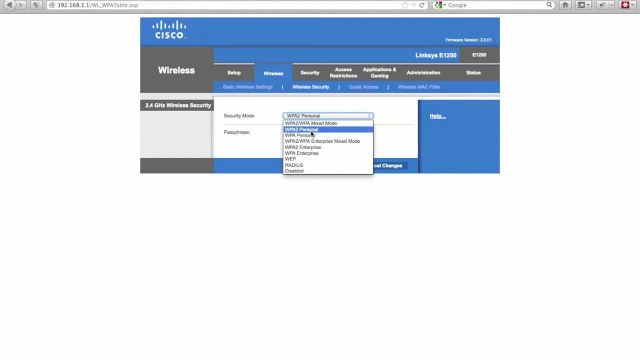 WPA is really Really the standard now. WEP was cracked a few years ago And in the purpose of this video you'll notice that the person who was got their information hacked was a victim of war driving And the reason they had that happen to them is because they were on a WEP network. 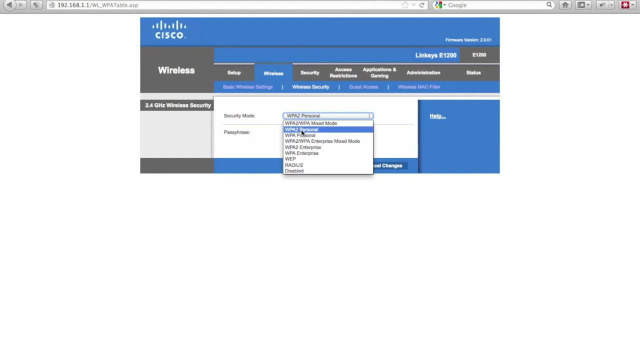 So I would highly recommend using a WPA or WPA2.. WPA2 has a little bit more of an encryption strength to it, And the benefit of that is it allows you to just type in a password- There's really no hexadecimal characters or anything like that- And you'll notice that RPA2 has a lot of. 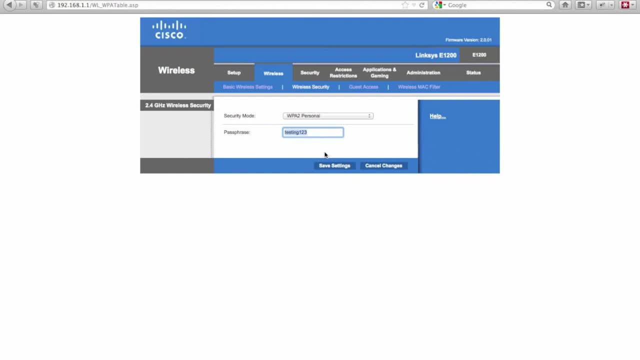 password is testing123, but you know you can really make it anything: my home network or virtually any password, anything that's easy for you to remember and it the encryption strength on WPA is a lot greater than WEP and you know I would highly recommend that over. I would highly. 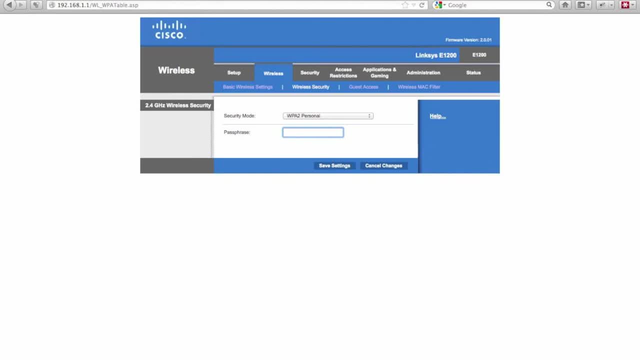 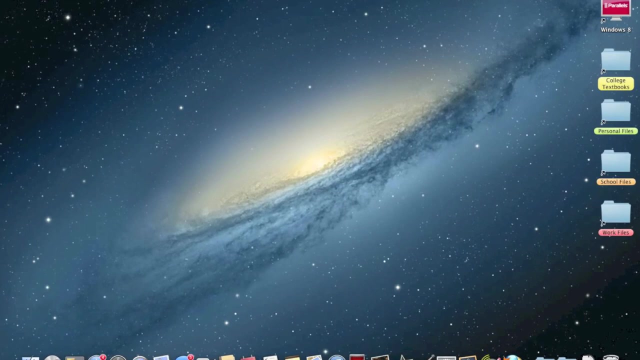 recommend WPA over WEP, and once that's done, you'll hit save the router, go through a little configuration and then it has saved the settings. and now let's take a look at how to connect to our newly created network. so, as you can see, we're using Mac. for this example, Windows is going to be. 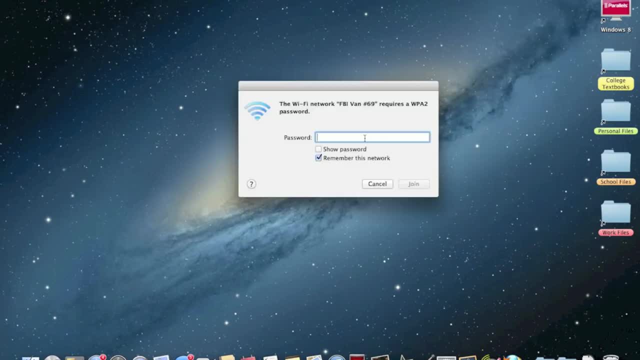 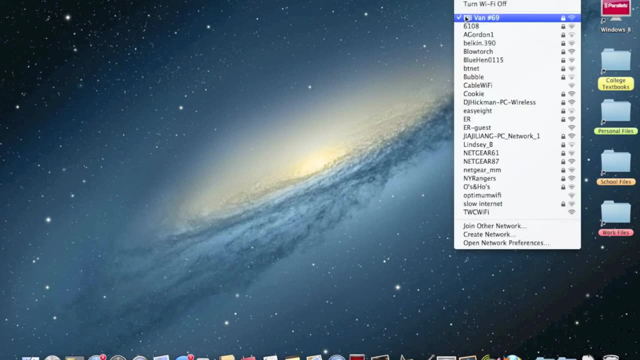 a little different, but you want to find the wireless symbol on either the finder bar or on the start menu bar at the bottom for Windows, and you want to find the wireless access point that you're going to be connecting to. once you do that, you just type in the password and now you can see. 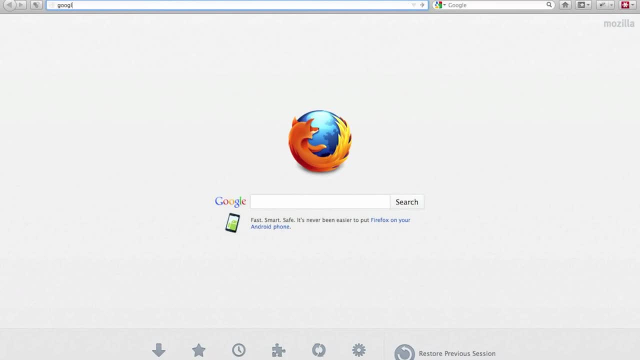 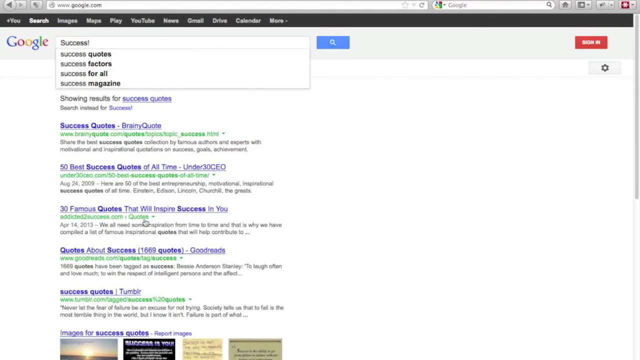 that we're connected and then, if we go over to the internet, we'll do a simple Google search, we'll go to googlecom and then we'll type in success and, since we are seeing web content destruction displayed, you can see that you've now connected to this wireless network. congratulations, my name.